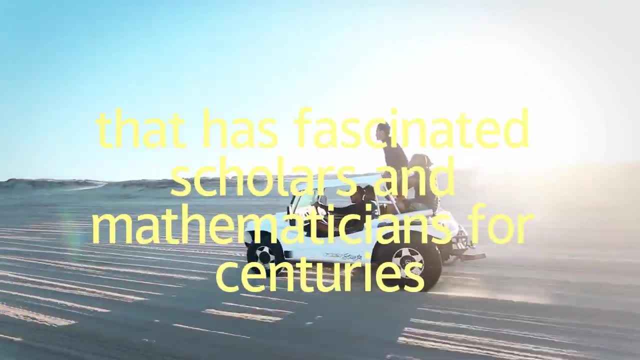 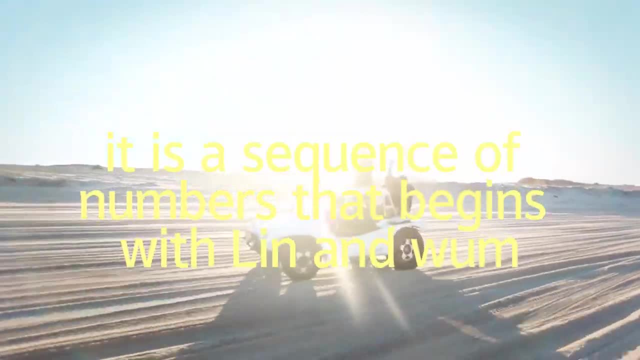 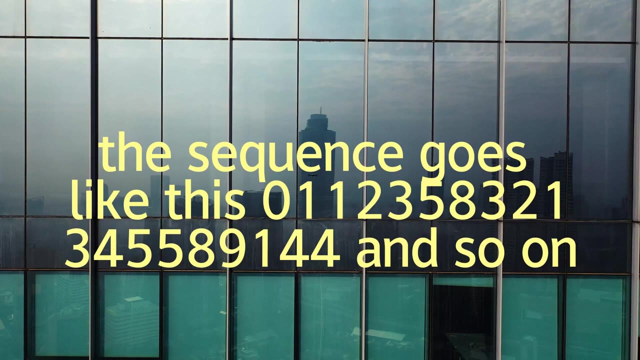 The Fibonacci sequence is a mathematical concept that has fascinated scholars and mathematicians for centuries. It is a sequence of numbers that begins with 0 and 1, and each subsequent number is the sum of the two preceding numbers. The sequence goes like this: 0, 1, 1, 2, 3, 5, 8, 13, 21, 34. 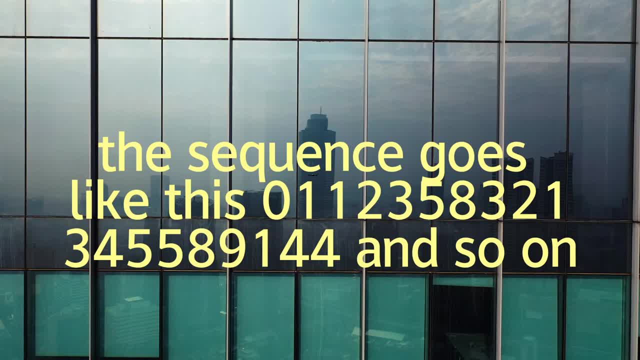 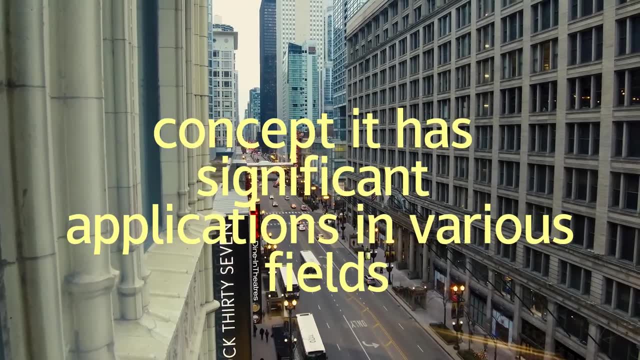 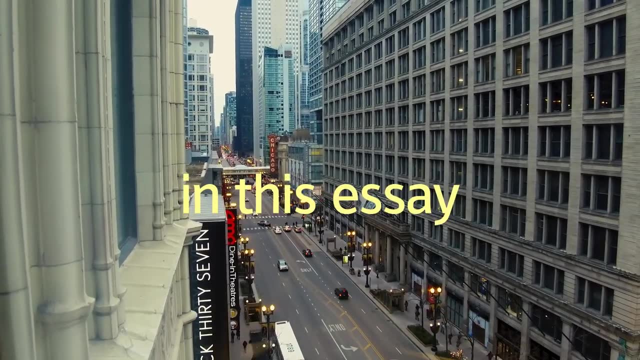 55, 89, 144, and so on. While the Fibonacci sequence may seem like a simple and abstract concept, it has significant applications in various fields, including mathematics, science, nature and even art. In this essay, we will discuss some of the best advice on the Fibonacci sequence. 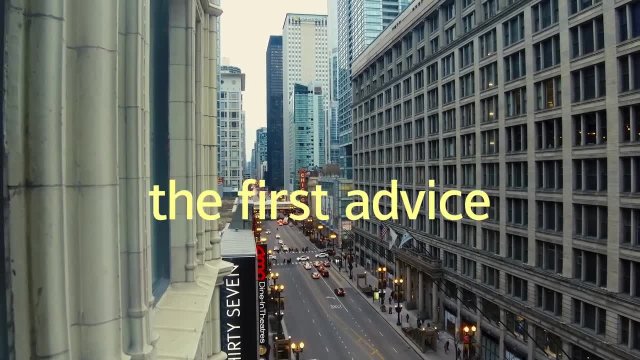 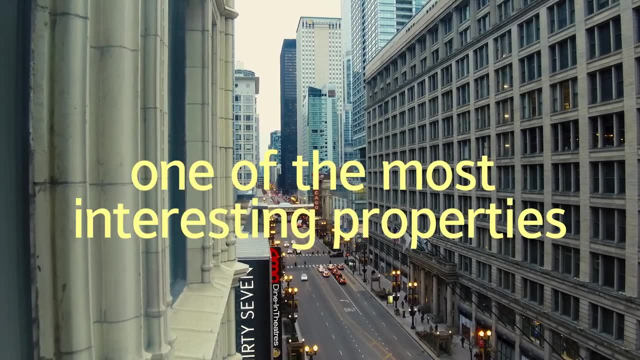 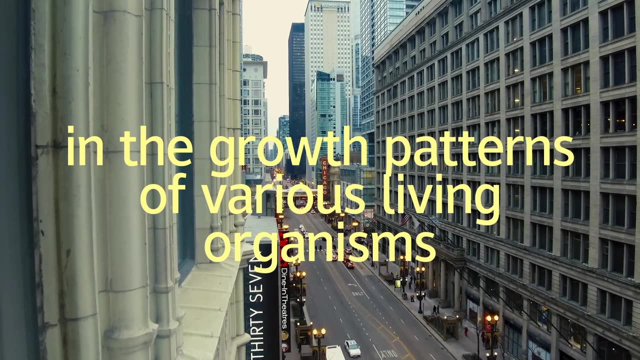 its properties and its applications. The first advice we can give on the Fibonacci sequence is to understand the Fibonacci sequence, its properties. One of the most interesting properties of the sequence is that it appears in nature, in the growth patterns of various living organisms such as flowers, shells. 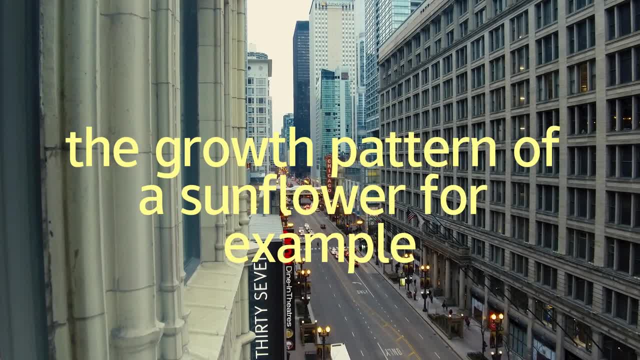 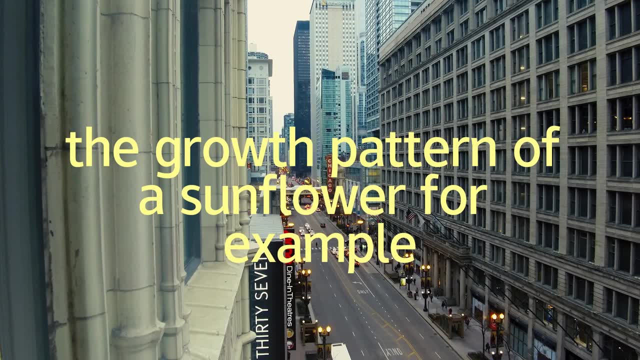 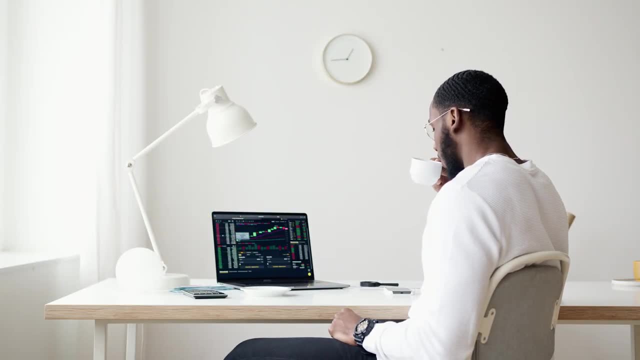 and pineapples. The growth pattern of a sunflower, for example, follows the Fibonacci sequence, with the number of spirals in one direction being a Fibonacci number and the number of spirals in the other direction being the next consecutive Fibonacci number. This pattern is not only 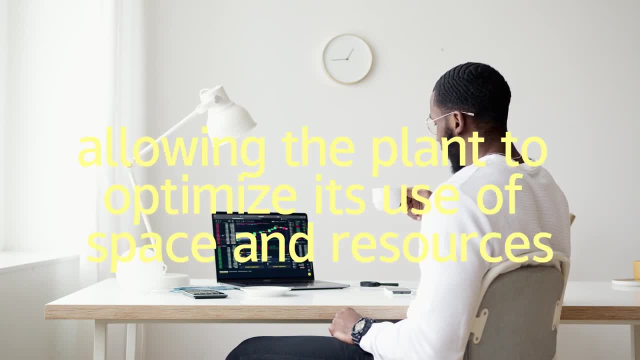 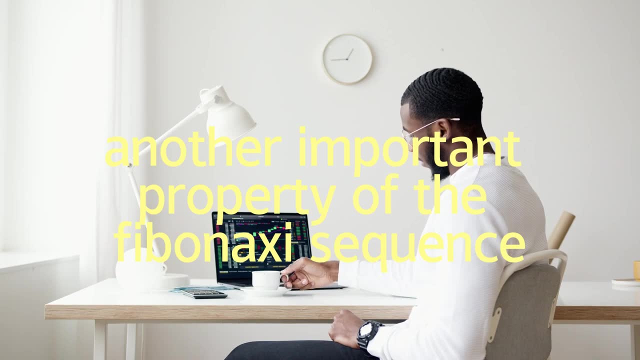 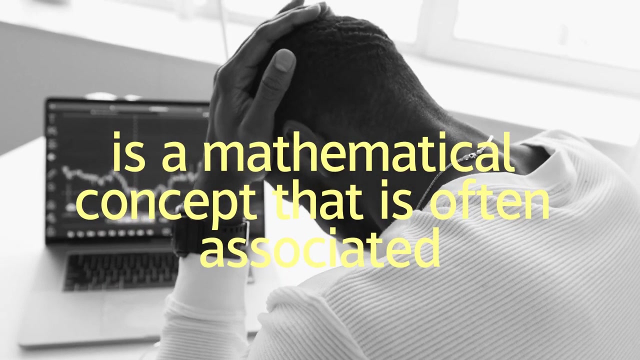 aesthetically pleasing, but also serves a purpose allowing the plant to optimize its use of space and resources. Another important property of the Fibonacci sequence is its relation to the golden ratio. The golden ratio is a mathematical concept that is often associated with beauty and 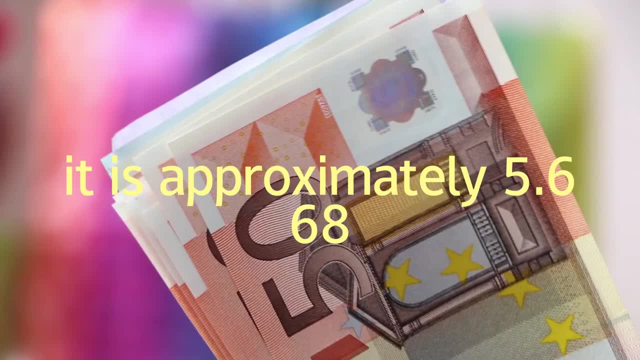 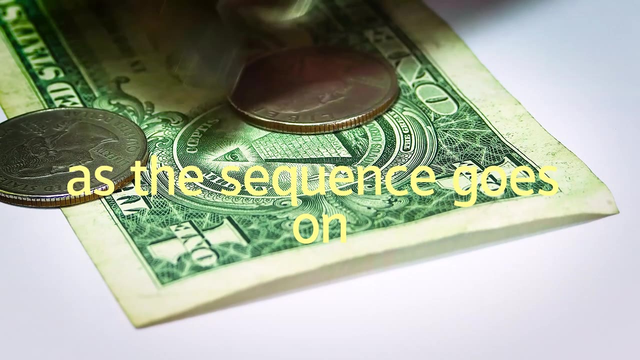 aesthetics It is approximately 0.618.. And it appears in the proportion of many objects, from the human body to ancient buildings. The ratio of two consecutive numbers in the Fibonacci sequence approaches the golden ratio as the sequence goes on. This relationship between the Fibonacci sequence and the golden ratio. 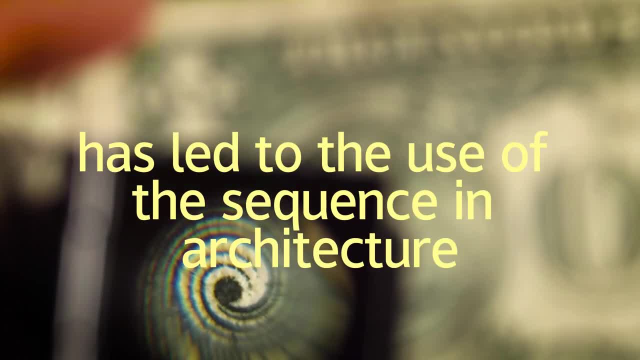 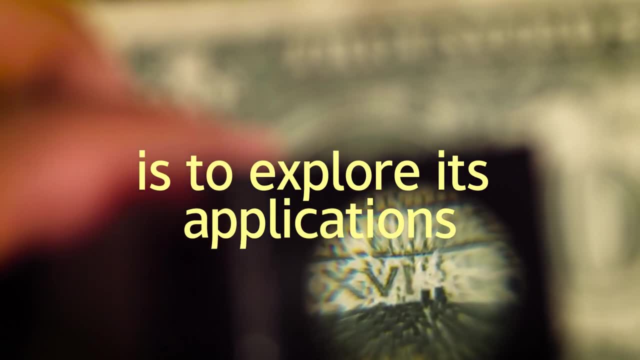 has LED to the use of the sequence in architecture, art and design. The second advice we can give on the Fibonacci sequence is to explore its attributes. The second advice we can give on the Fibonacci sequence is to explore its attributes. The third advice we can give on the Fibonacci sequence is to explore its attributes.